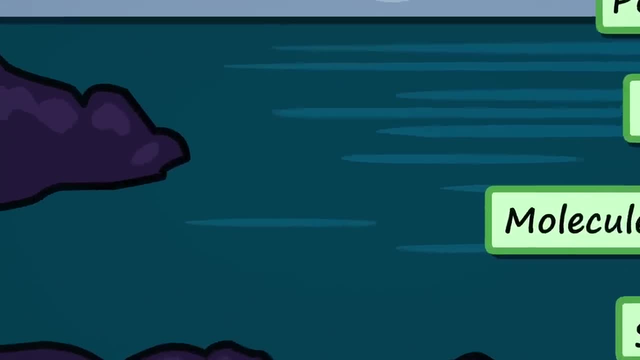 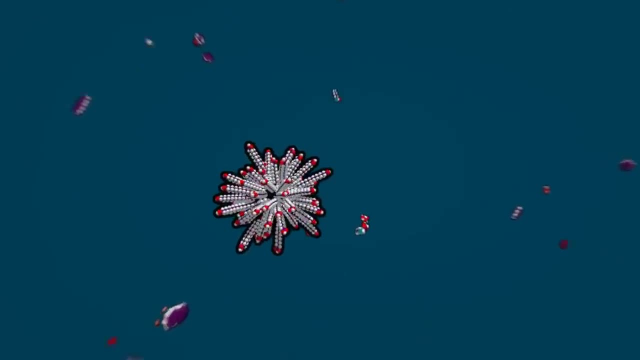 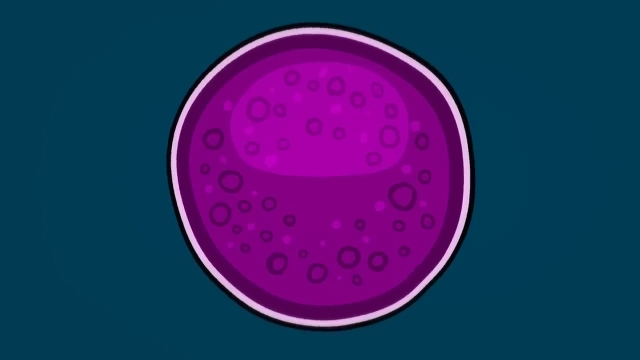 to living cells. He imagined the early ocean as a primordial soup, a rich collection of complex molecules produced by natural chemical reactions. In this soup, further reactions could take place, eventually producing life. At the time, Darwin's warm little pond and Oparin's primordial soup were really just speculation. 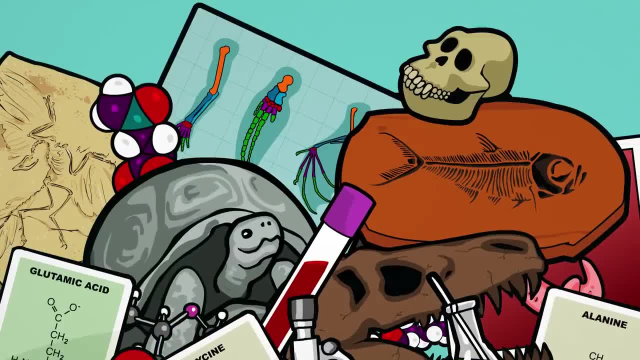 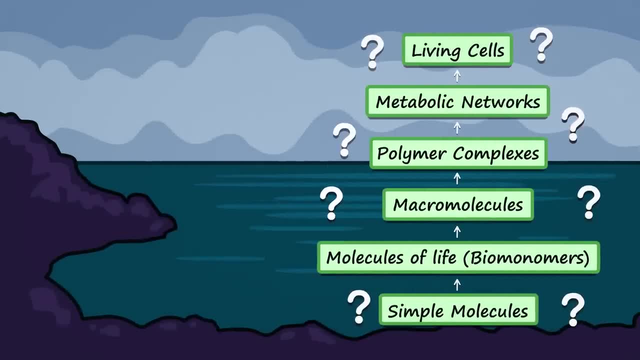 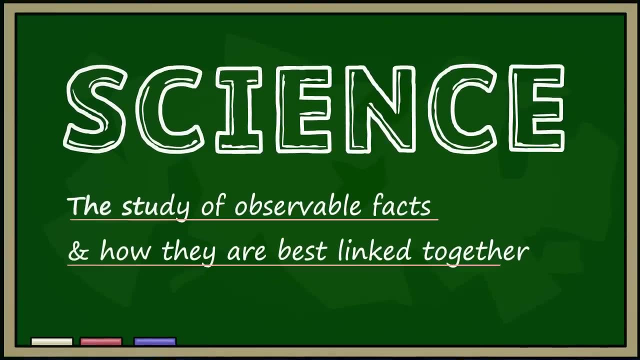 They were founded on a good understanding of chemistry and biology, but they could not be considered legitimate scientific hypotheses because no one had found a way to test or observe them. Science, after all, is the study of observable facts and an ongoing conversation about how those facts can be best linked together. 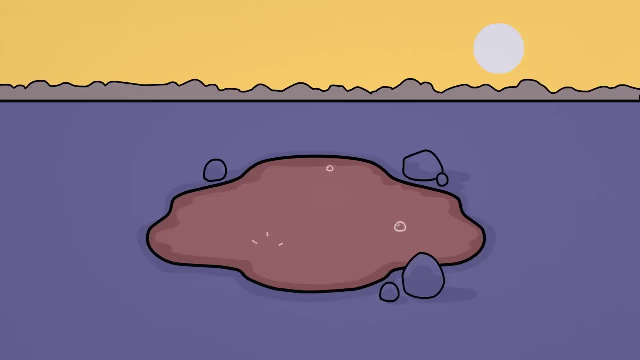 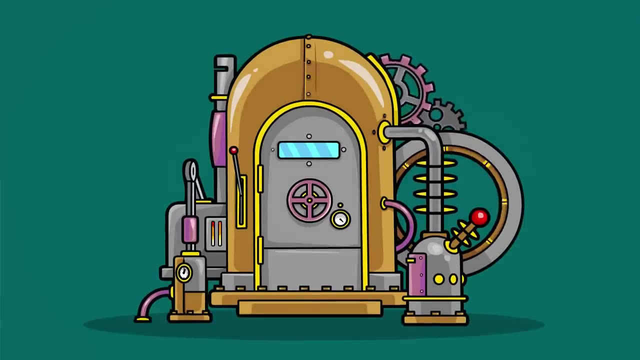 Chemical reactions like those proposed by Darwin and Oparin are not expected to leave an observable fossil record. Without either having fossils to examine or a time machine to travel back and observe what happened, how could scientists even begin to study the origin of life? 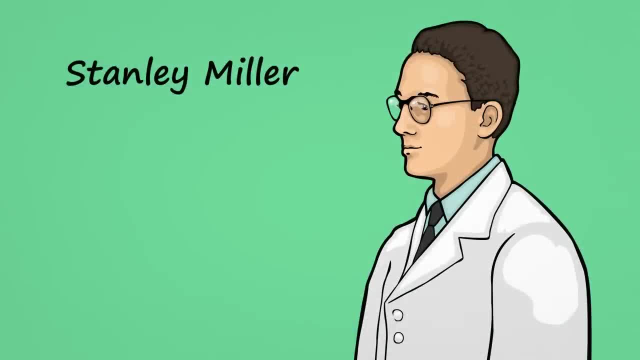 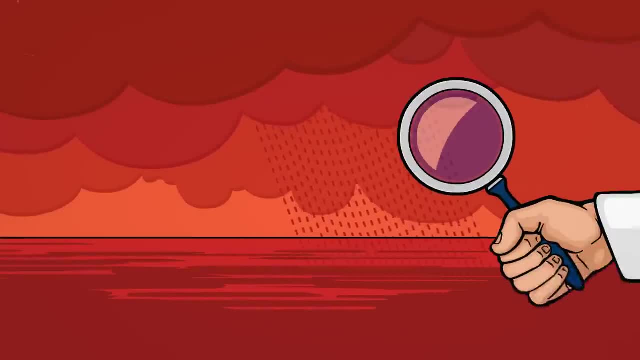 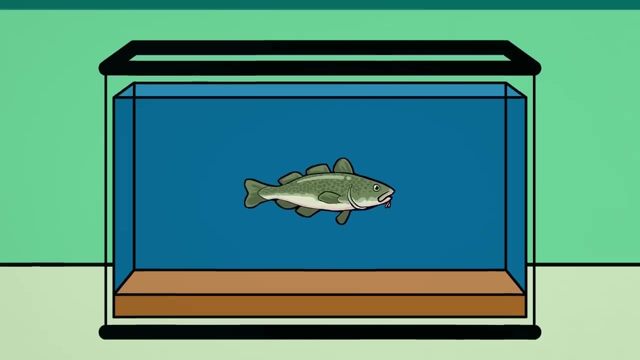 In the 1950s, Stanley Miller, then a graduate student at the University of Chicago, came up with an idea: We could simulate early Earth conditions in the lab and then carefully watch what happens. To study fish in the sea, set up an aquarium. 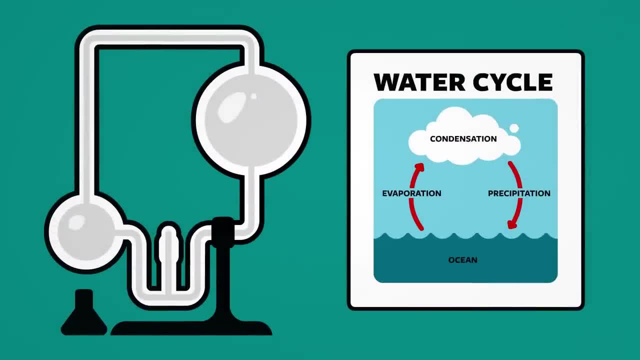 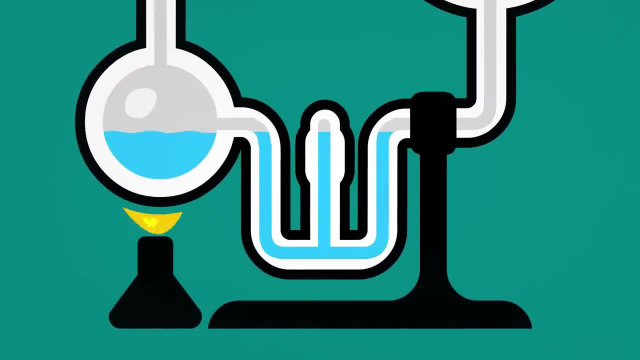 Working with his professor, Harold Urey Miller, designed an apparatus to simulate the ancient water cycle. Together they put in water to model the ancient ocean. It was gently boiled to mimic evaporation Along with water vapor. for gases of the atmosphere they chose methane. 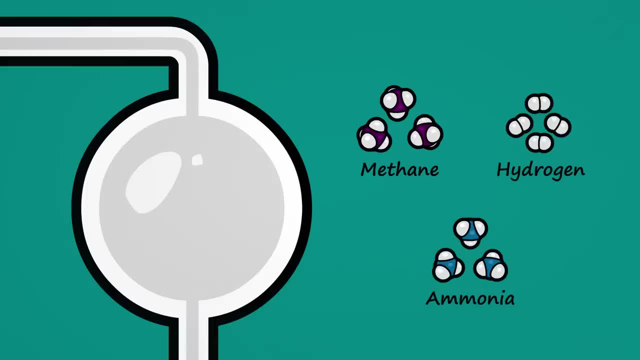 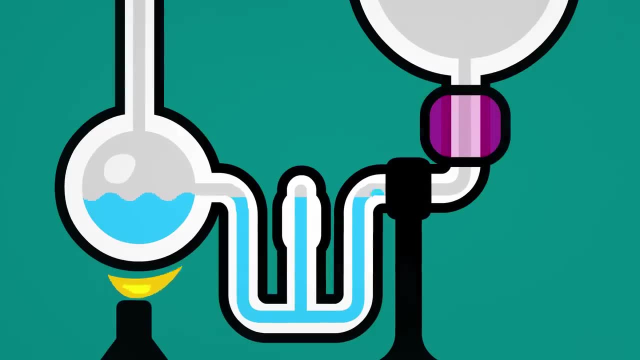 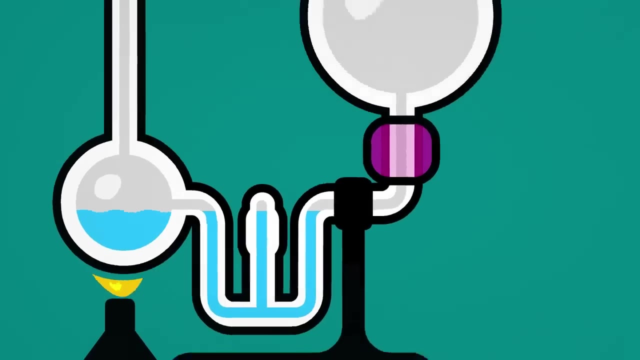 hydrogen and ammonia. These are simple gases which scientists at the time thought were probably abundant on the ancient Earth. What is the answer? They added a condenser to cool the atmosphere, allowing water molecules to form drops and fall back into their ocean like rain. The ancient Earth would have had many sources. 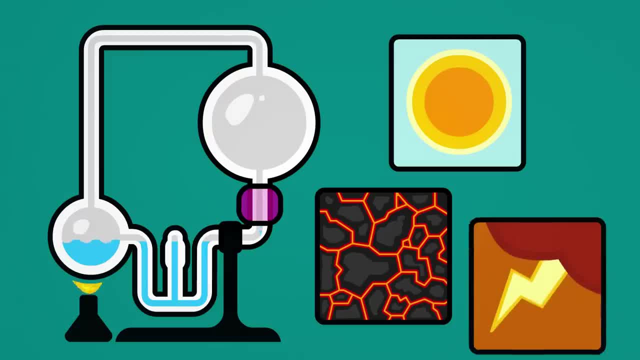 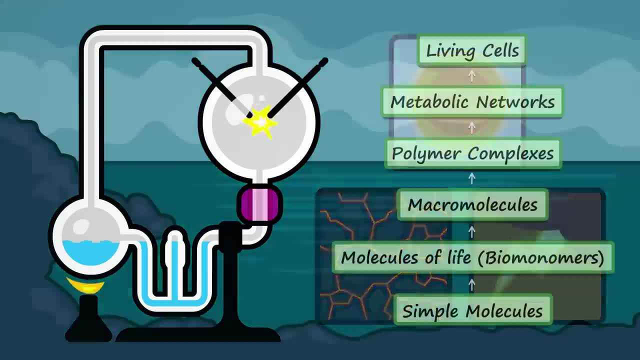 of energy—sunlight, geothermal heat and even thunderstorms—so they added sparks to the atmosphere to simulate lightning. The goal of the experiment was not to create life, but to simply test the first step in Oparin's model. 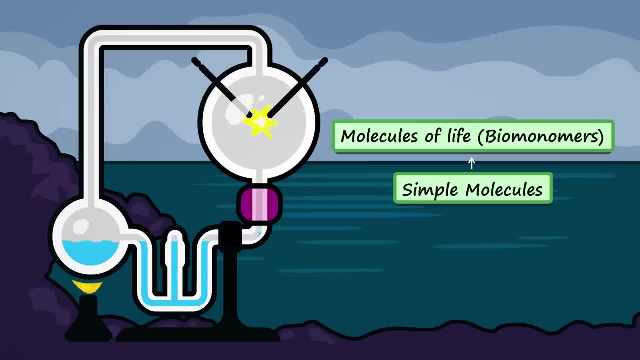 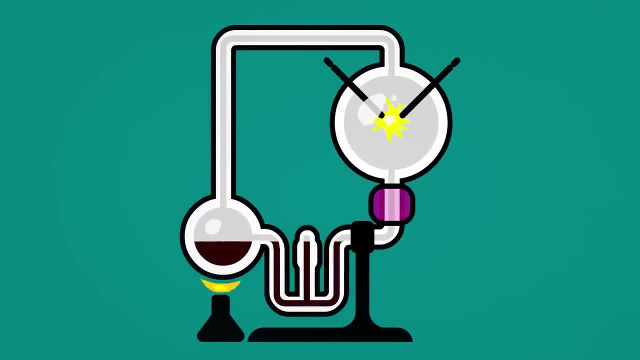 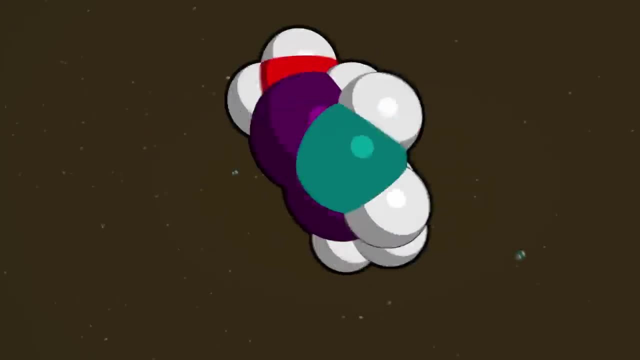 Can simple chemistry Naturally give rise to the complex molecules of life? After running the experiment for just one week, their ocean became brownish-black. Careful analysis revealed that, through a series of reactions, many complex molecules had been produced. Among these were amino acids—special molecules of life that we once thought could. 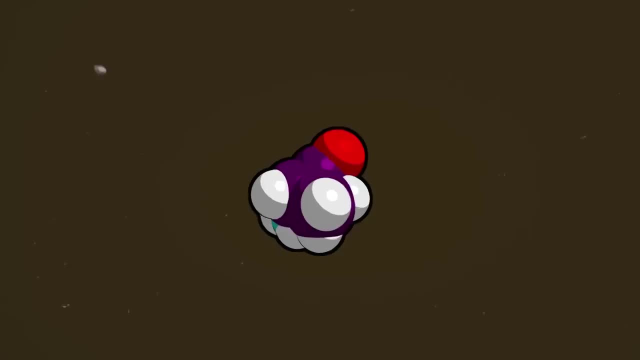 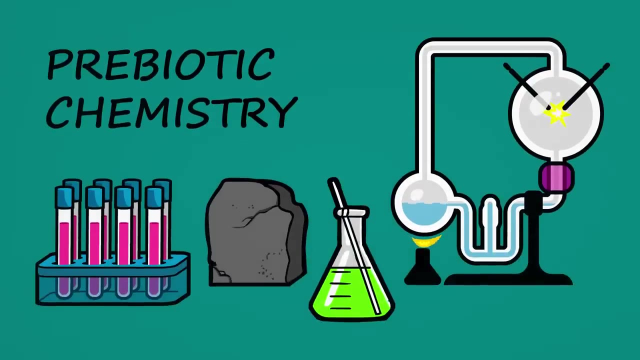 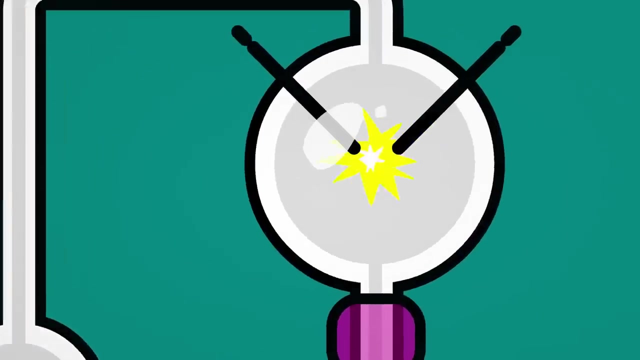 only be built inside the bodies of living creatures. This was a pivotal breakthrough in science—so significant, in fact, that it was impossible for scientists to predict what would happen next. Scientists don't know for sure if the gases used by Miller really were the most common. 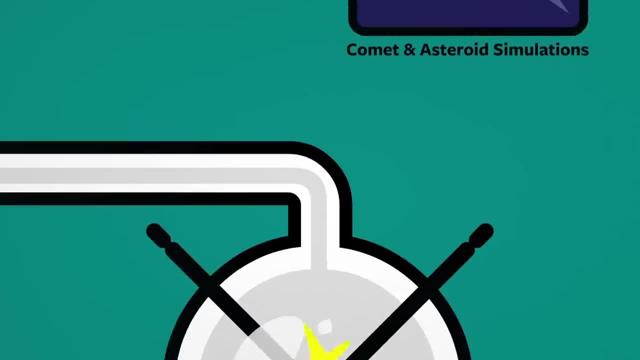 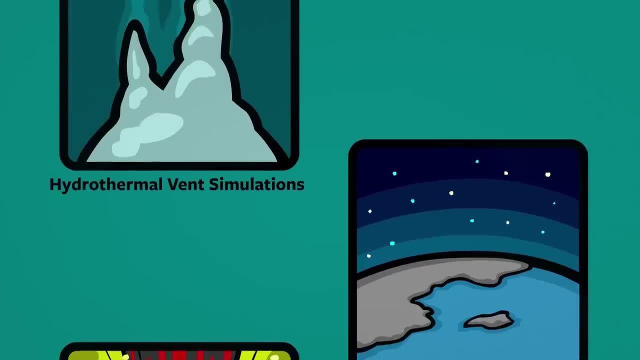 gases of the ancient Earth. Because of this, many experiments have since been done, showing that the molecules of life can form in a wide variety of environments with different starting chemicals and different sources of energy. Sugars, lipids and amino acids have even 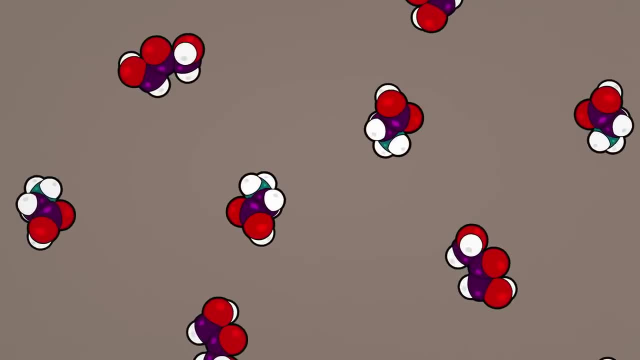 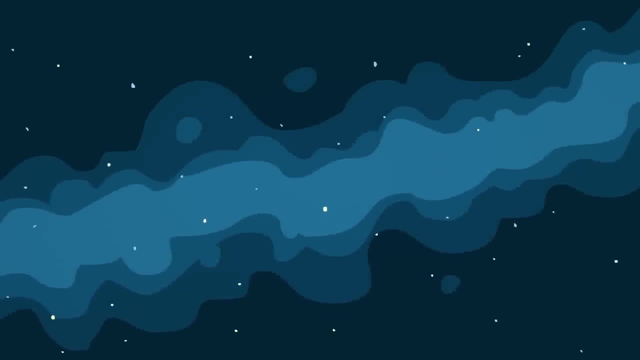 been found on meteorites. What is the answer? Can simple chemistry? This suggests that the molecules of life formed all throughout the ancient solar system and may be forming right now in other regions of our galaxy. Together, these discoveries tell us that Oparin's primordial soup and Darwin's warm little 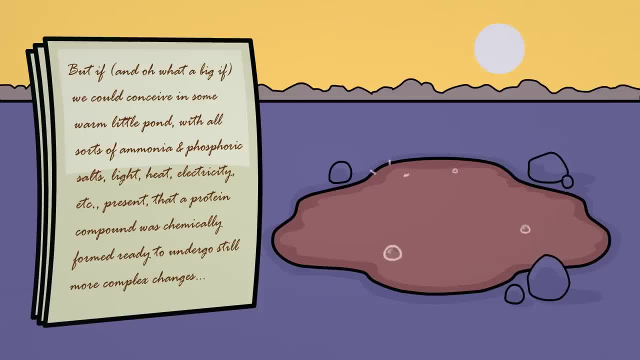 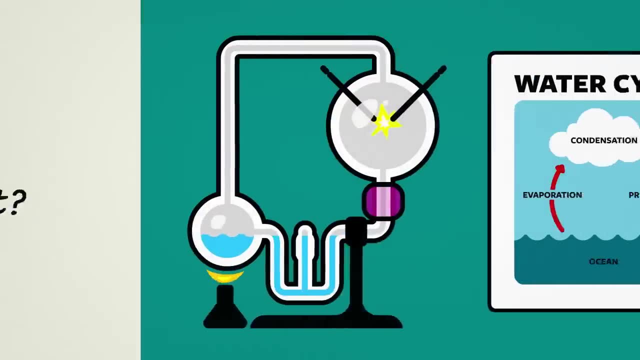 pond could have easily existed in one way or another on our ancient planet. So, to sum things up, what was the Miller-Urey experiment? The Miller-Urey experiment was our first attempt at simulating ancient Earth conditions—in this case, the ancient Earth. 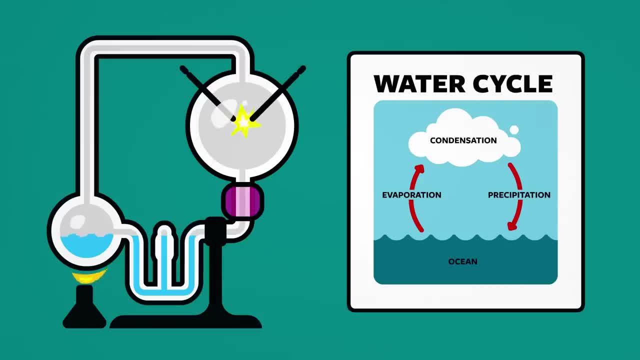 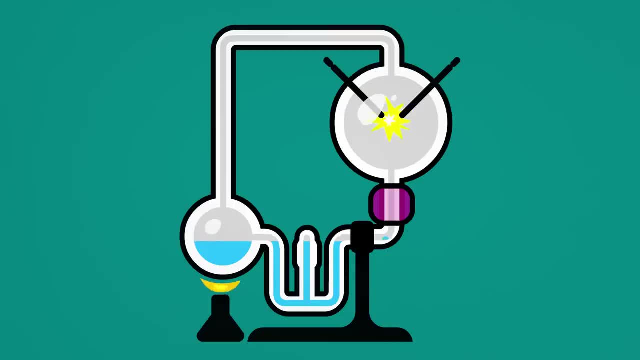 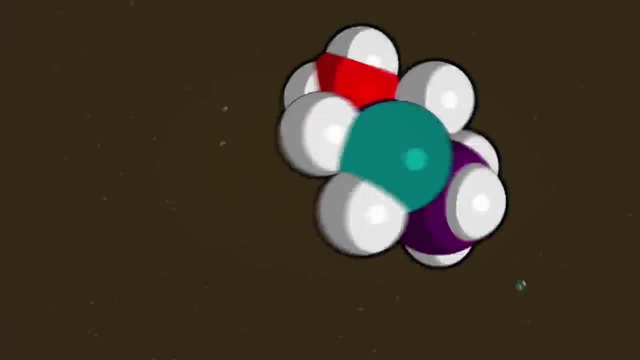 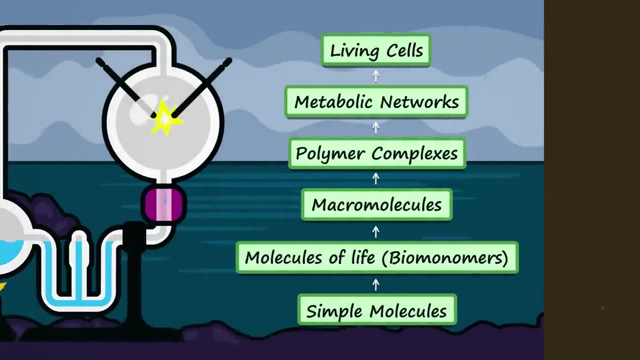 The Miller-Urey experiment is significant for two main reasons. First, though it was not a perfect simulation of the early Earth, it clearly demonstrated for the first time that biomolecules can form under ancient Earth-like conditions. Second, the experiment took what was once mere speculation—the idea that life may have emerged from chemistry—and 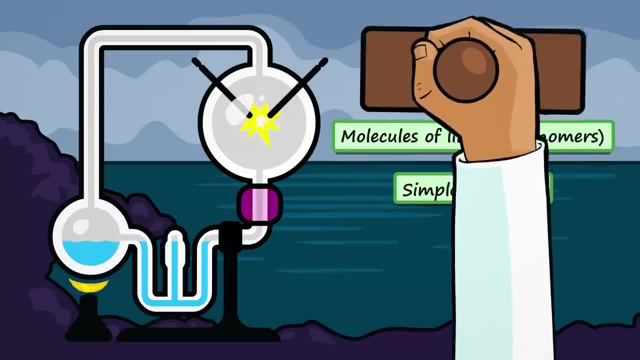 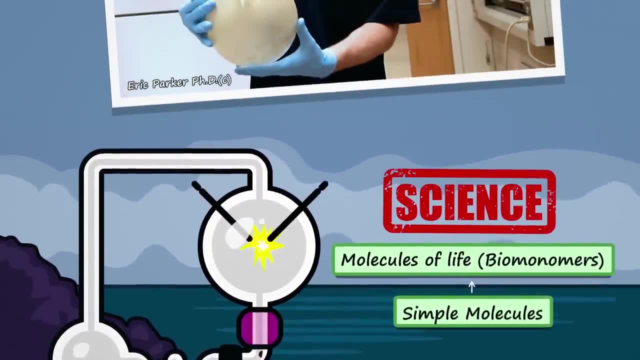 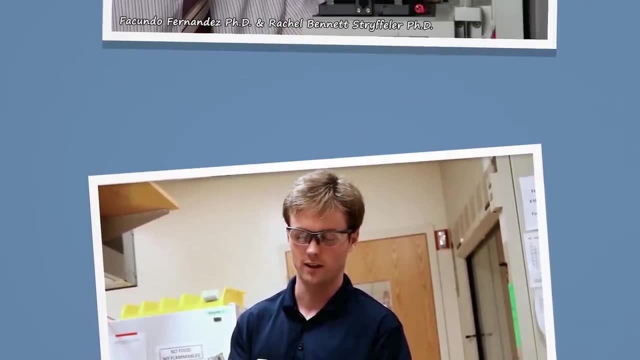 transformed a portion of that speculation into legitimate, testable science. Many questions remain to be answered about the origin of life, but scientists from many nations and many fields of study are now following Stanley Miller's lead. They're finding ways to turn those questions about the origin of life into testable scientific hypotheses.